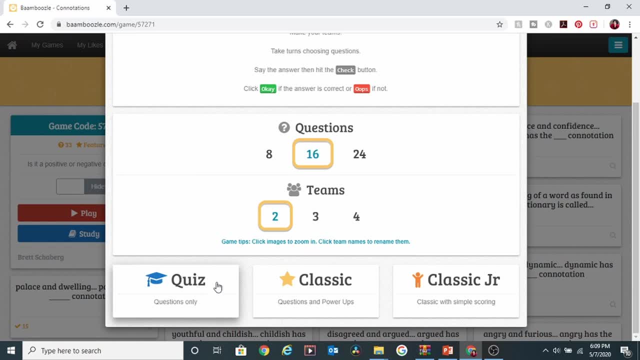 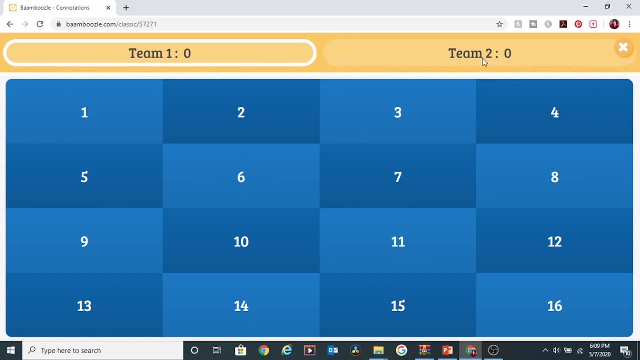 And every game tells you how it's played and how many questions you can set it up to have- have eight, 16 or 24, and how many teams- And the classic is the, usually the one that I choose, And you'll see why. it's a really a lot of fun. And let's say you have two different teams. 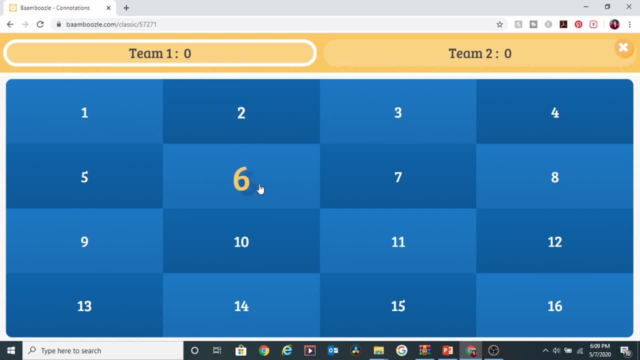 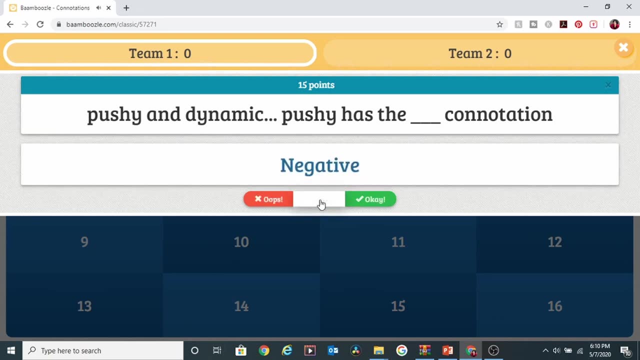 and you. what you're going to do is establish who's going to be on team one and team two, and team one goes first. they choose a number And let's say, for example: the question is push and dynamic, pushy has the connotation. You click on the white and that is the answer that 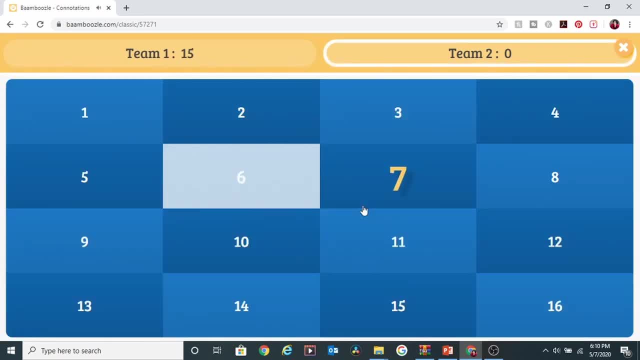 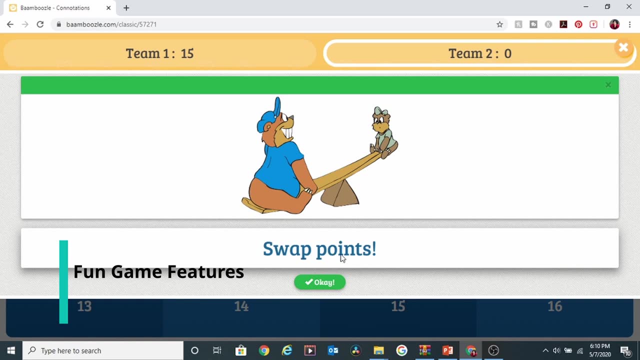 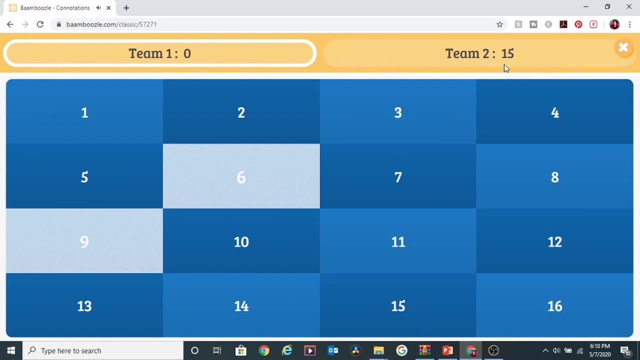 they have to choose. Is it negative or positive? If they get it correct, you click okay And they get a point. Now here's the thing about this game: It's it seems like it's normal, but then when team two goes, they have the choice whether to swap points or not. So that means that team 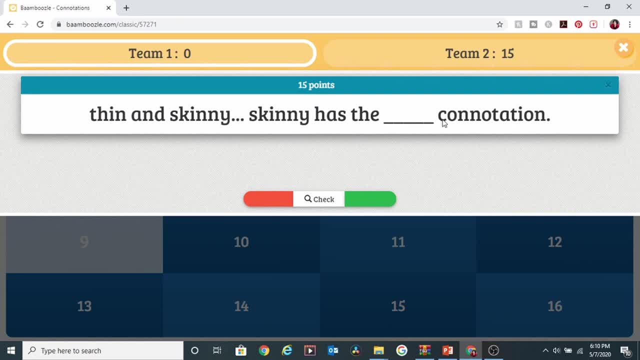 two gets to steal 15 points from team one, And then, um, team one is left with zero points. Then it goes back to team one. You click on white so that they determine whether they're going to win or not, And then you click on the white and that means that they're going to. 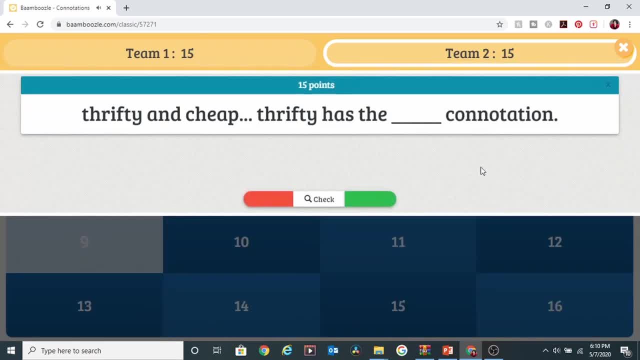 that's correct or not. If they say that it is correct, they get a point, and so forth. If they get it wrong, you're going to click on the red button, and the red button signifies that they got the answer incorrect and they get no points for that. But what they really like about it is: 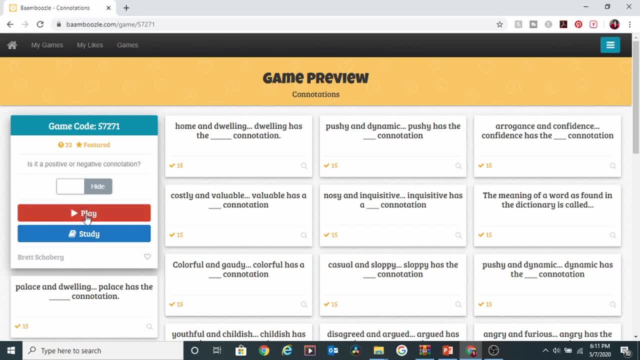 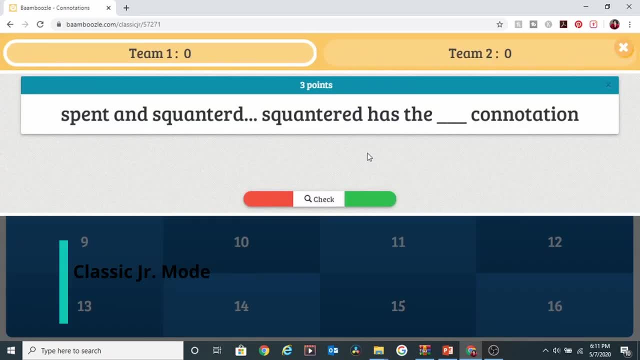 that they don't know what's going to happen. They may get the point or they may have the choice whether to do something different. And, um, what's really nice too, is that for the classic junior. if you decide to do that, it's similar. 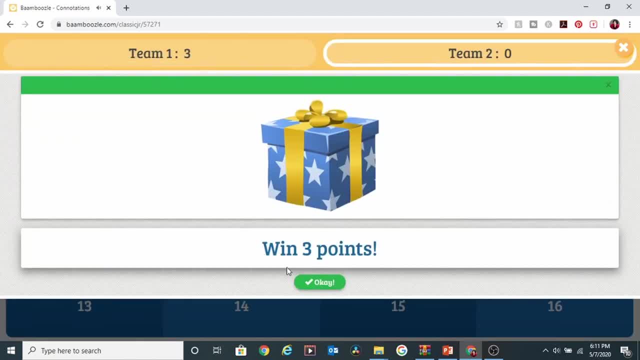 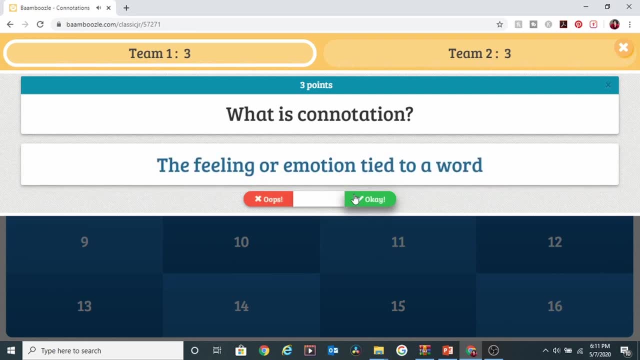 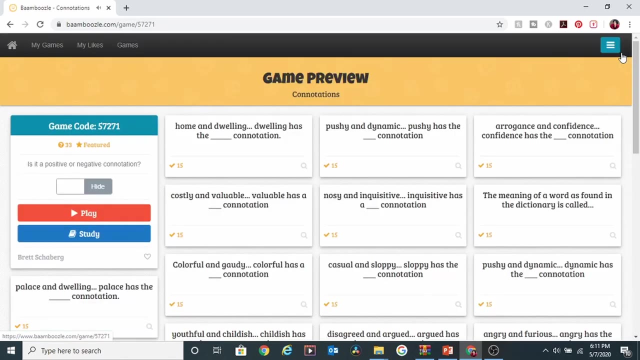 to the other one, except that there's no um hidden agenda. like you know where you can swap points, It's just you win the point straight through. So if you have students who are a lot more sensitive and will be upset by losing their points- I teach middle school, So my students tend 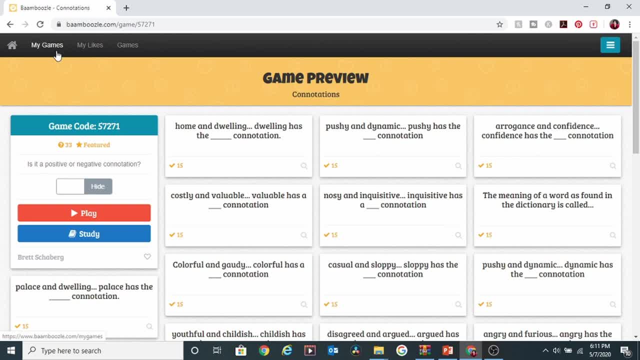 to really like having that option of- oh my goodness, like what's going to happen, And they like to get each other back And it's a lot of fun, like a lot of healthy, playful competition. And here is like a list of all of the 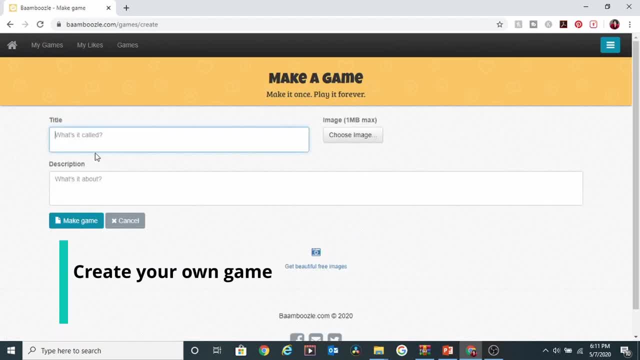 like again the game preview. If you really like a game, you can save the game code and you can go back to another time. Now this is for like. if you're going to make your own game, so you create your game, And I've been using a specific uh story with my students. 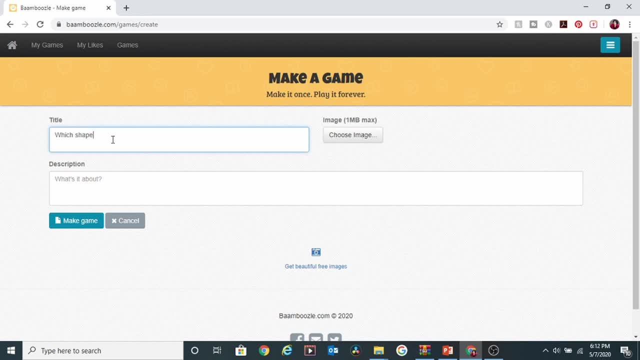 um called Trino's choice, And so here is where I have the option of creating my own game If I happen to find one that's not already made for specifically I want to do with my students, So in this box you're going to actually find the title You're. 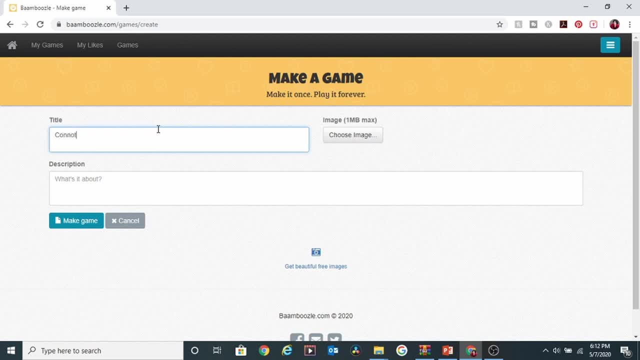 going to write up a title and in the next box you can create an image. I didn't, but that's just so that you can uh make it specific or link it up to, you know, the game that you're playing. 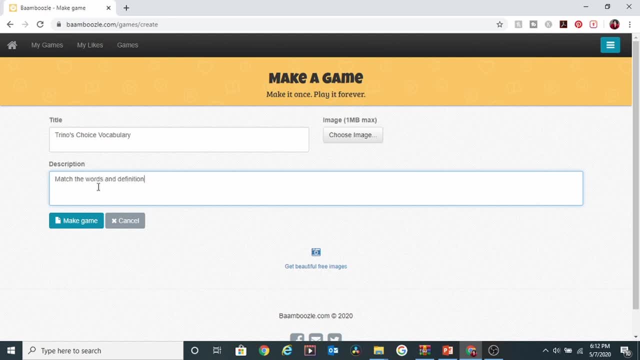 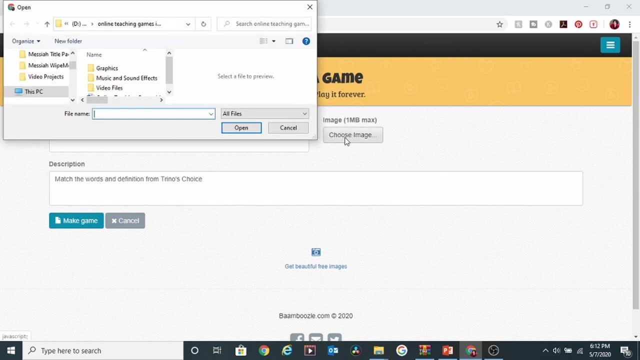 And then there's the actual game, And here you would type in the description: Um, and that's a good way for you to remember, um, what the game is about. or, if you decide that you want to create a game, you can create a game. So, if you want to create a game, you can create a game. 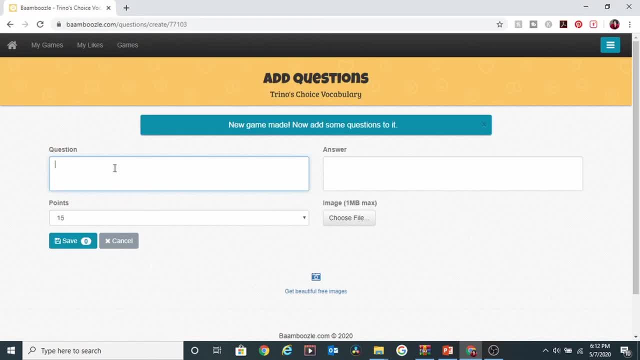 If you want to make your game public, then other people can actually see the game as well. Um, but I usually keep mine private. And then here's where you type in the questions and you can determine. you know you can ask any type of question, whether it is a yes, no answer. 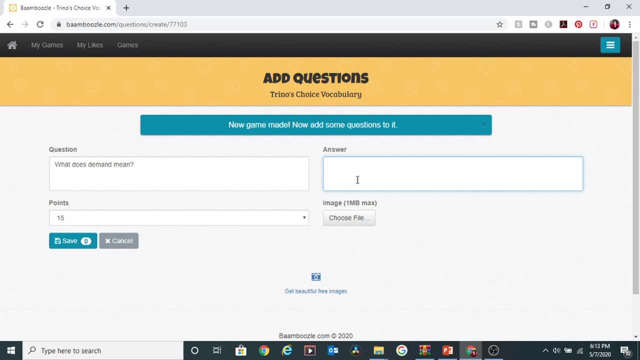 or they have to say yes or no, or if it's correct or incorrect. And here's where you actually write the answer to the question that you have chosen, And then you can type in the questions and you can ask any type of question, whether it's a yes, no answer. 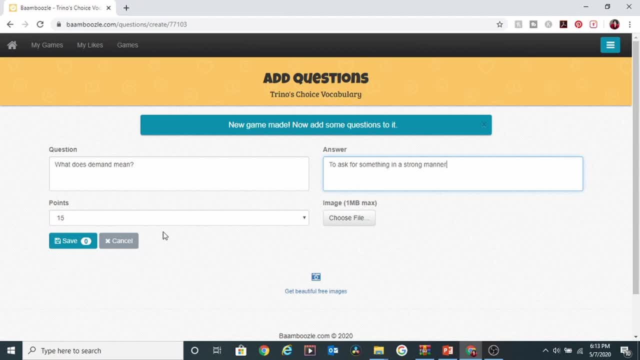 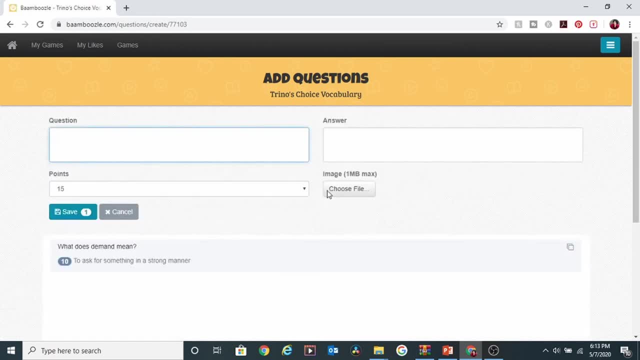 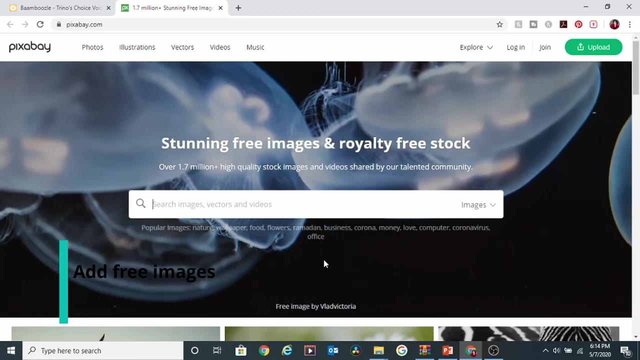 you can denote how many points. So any questions is a little bit more difficult or challenging, I usually increase those points And if it's easier I'll give them less points. And then let's say that you want to add an image. You can click on this button and then you can. 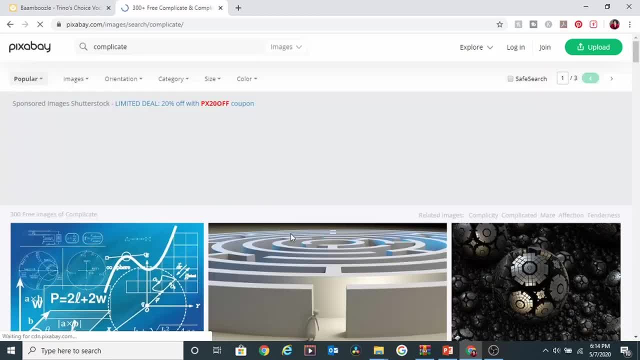 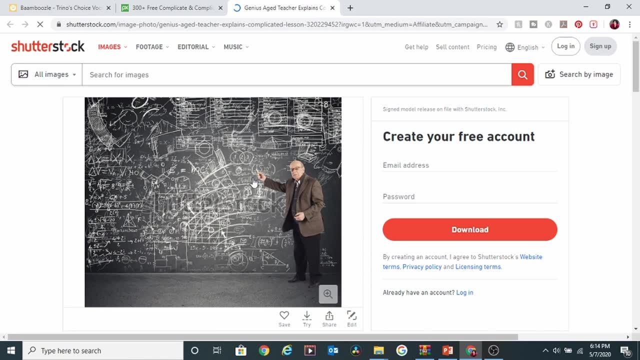 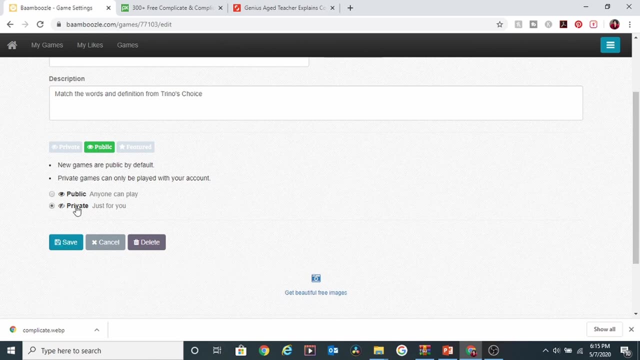 find royalty free images that connect with um, what you are doing for your class, for each of the different questions or for just the game. uh, topic in itself. You can make it public or you can keep it private. I keep it private at first because I like to test. 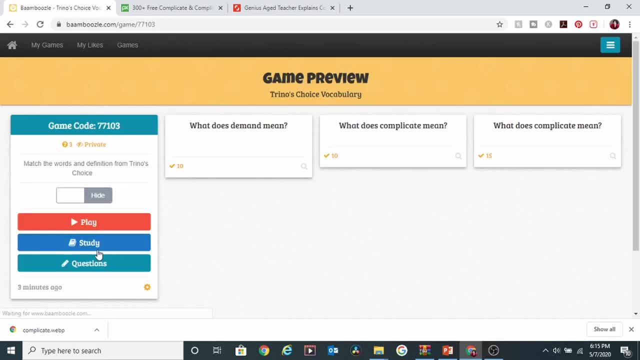 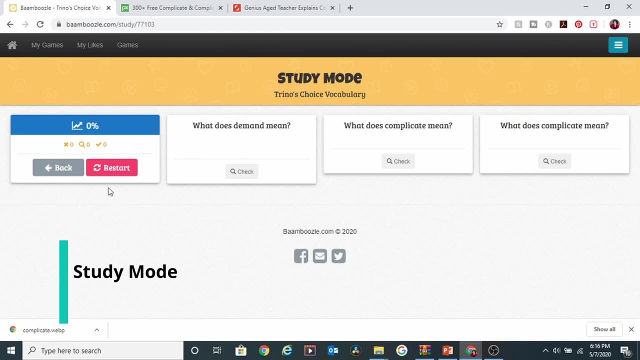 it out with my students And if they enjoy it and there aren't any hiccups, then I'll change it to private to public. This is the study mode function. Usually I'll start the class with a study mode so that they can practice through it right before they play the game, so that the game 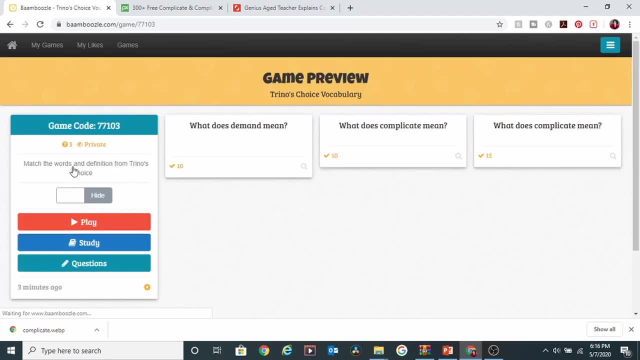 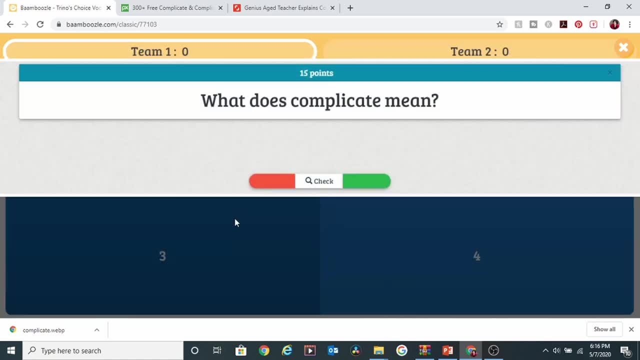 is something that they're familiar with already. Then for the play option, again it's your. what's really nice is that the game is never the same, Even if you choose, let's say, the, the version, one type of version, the second time you play this. 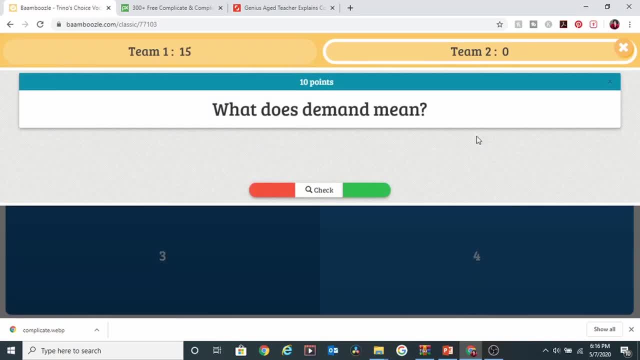 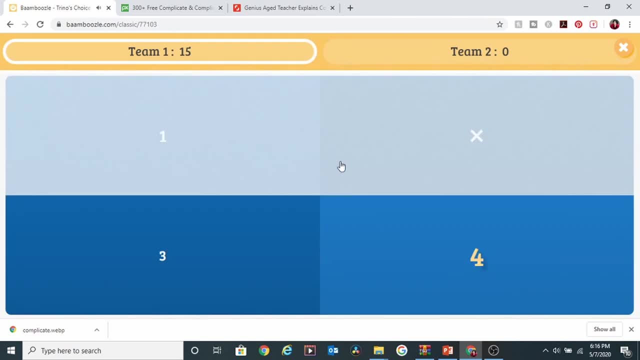 again. if they say, oh, let's play it again, it won't ask the same questions in the same order And they'll change things up because you know, question number one might ask them to swap points with team two, but on the second round, question one might not do that. So that's one of the features. 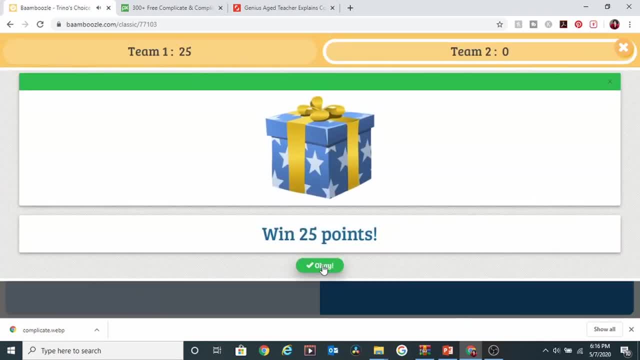 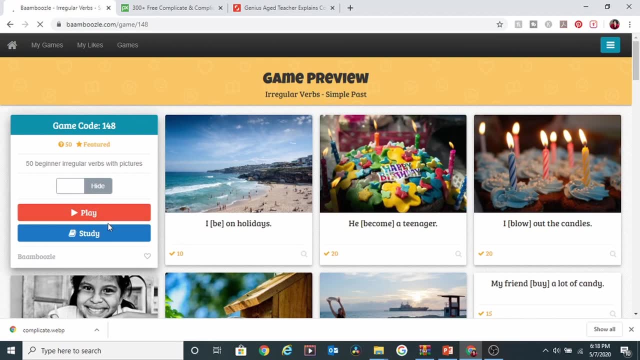 that I like about bamboozle, because you never know what's going to happen. You can assign these to your students individually, So I think that's a great way to get the students to be more aware of their homework for the week or class time. 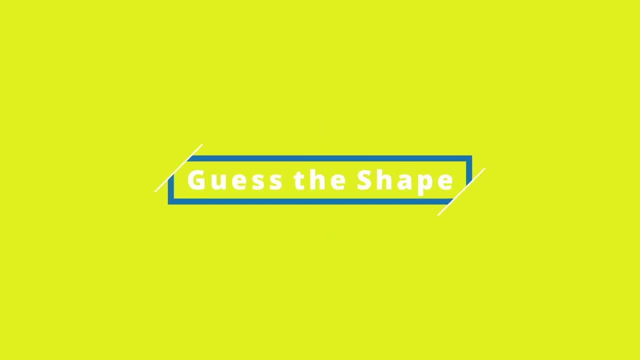 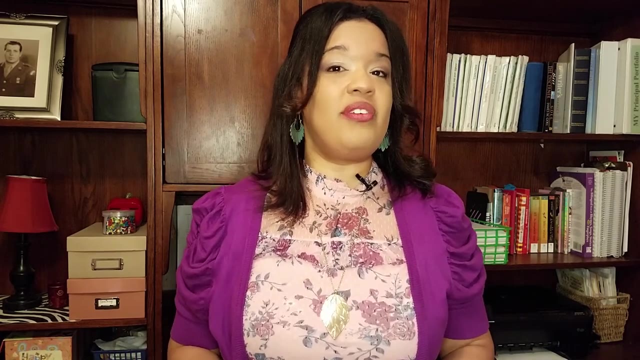 And it doesn't necessarily have to be in a game mode. The second game is called Guess the Shape, And by the looks of it it may look like it's tailored only for elementary students, but after I show you what you can do with it, you can tailor it to any age and grade level. 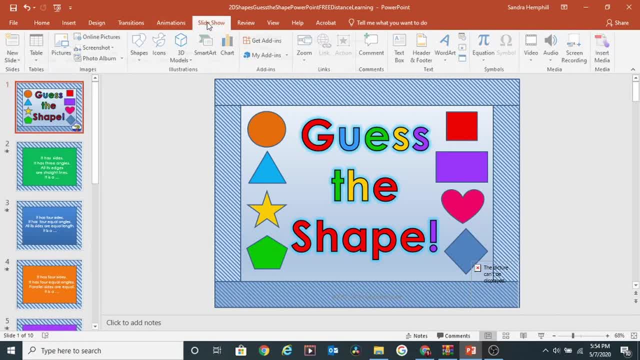 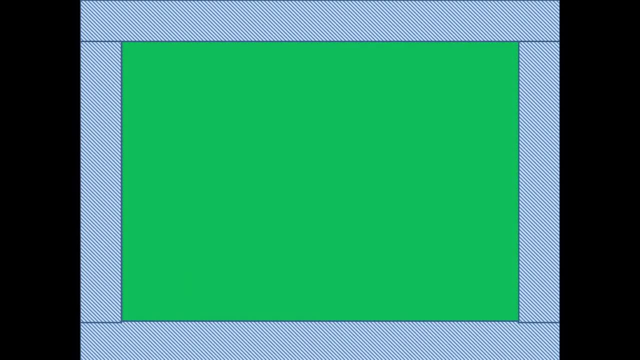 The reason why I love Guess the Shape so much is because this game can be used during the beginning of a class just to wet your students appetite, to get them curious about what they're doing. It could be part of a review and it can also be an assessment. 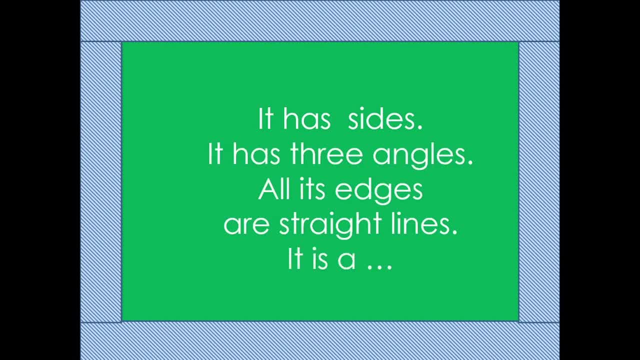 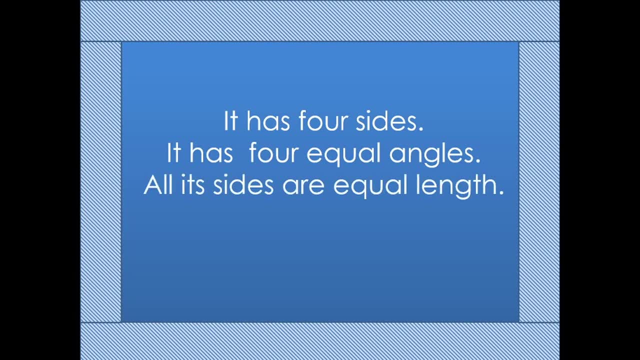 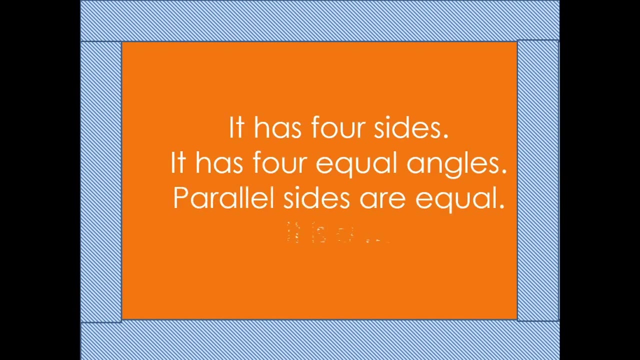 Essentially what it is is that you are clicking clues to something that they have to guess what that is. So, for example, the second one is it has four sides, It has four equal angles, All its sides are equal to, And then if they guess that it's a square and it just keeps going on and on every slide is a different color denoting that it's a different item that they're going to have to guess.